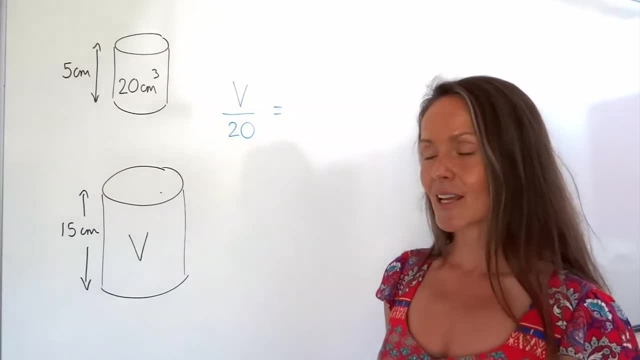 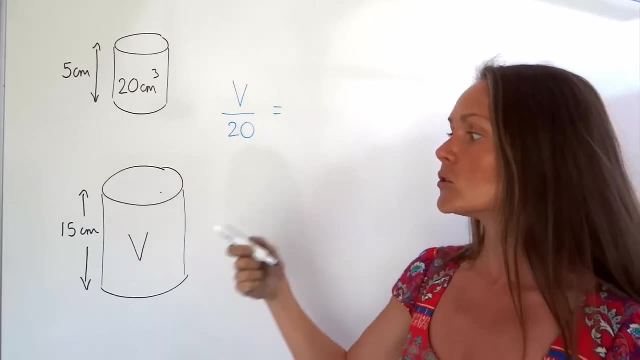 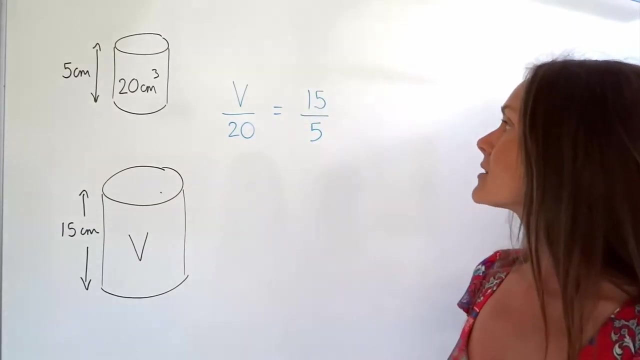 put that equal to the sides divided in the same way. so remember, we put the larger cylinder as the numerator and the smaller cylinder as the denominator. we do the same when we're looking at the lengths, so I'll go for 15 on top and 5 underneath. okay, so it doesn't actually. 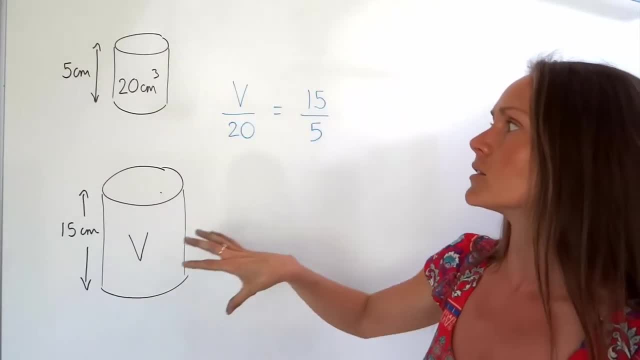 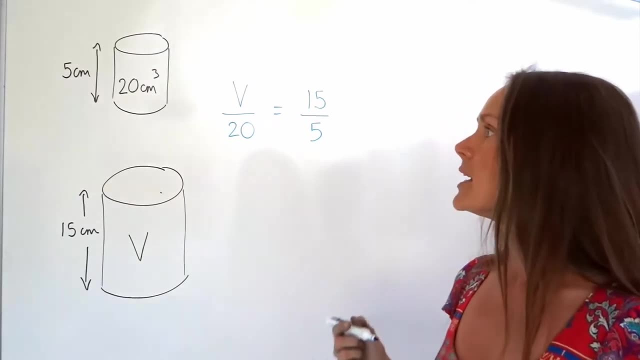 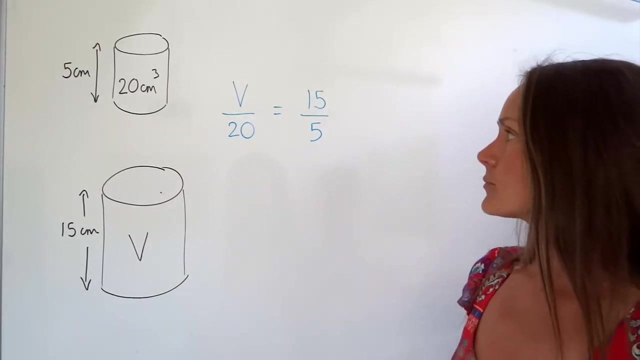 matter which way you divide these. okay, you could do it the other way around if you wanted to and you get the same answer. but it just makes your equations in general a bit easier to solve. if you keep the unknown as the numerator, that's all okay. so I'm going to continue with this question. I know 15 divided by 5 is 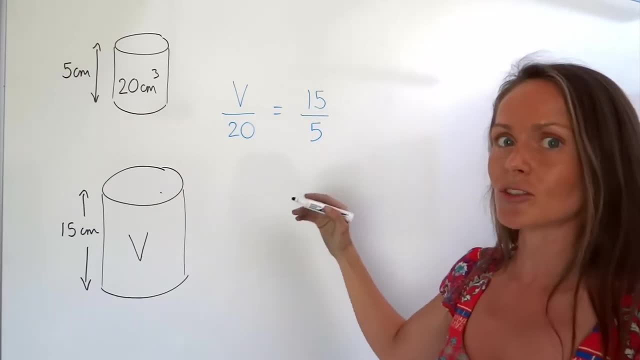 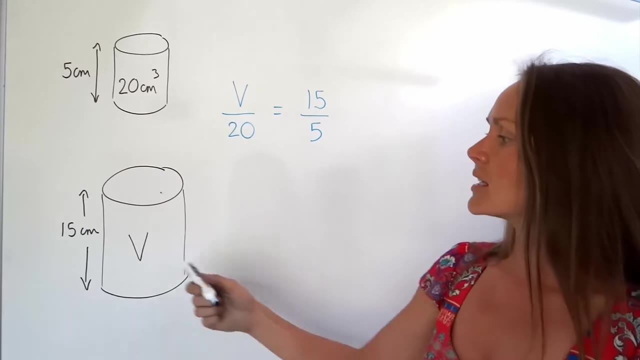 3. I'm just going to leave it like this for the moment, just so you know what to do in some of those harder questions. so the next step is to look at the units of our answer. the answer is volume, which will be in centimeters, cubed like this: 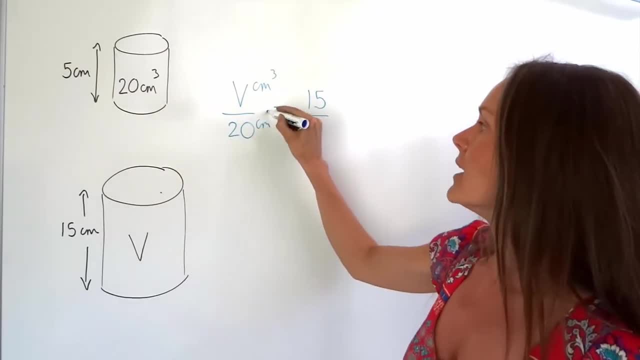 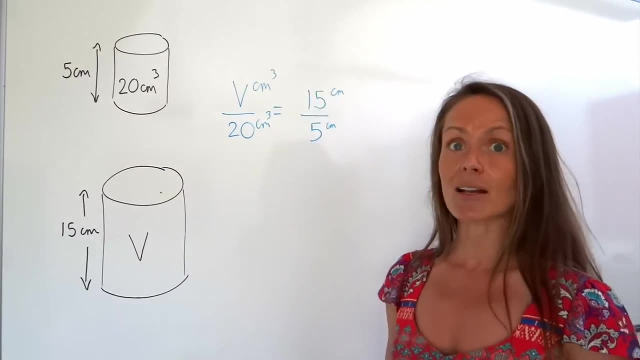 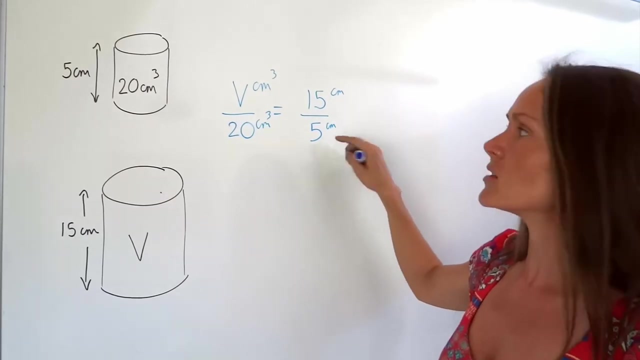 one. this one is already in centimeters cubed and the lengths are in centimeters. we need to make sure the units of all these numbers are the same as our answer. so, centimeters cubed. well, this one's alright, this one's already done, but these two are in centimeters, so we need to make sure we cube this side first. so 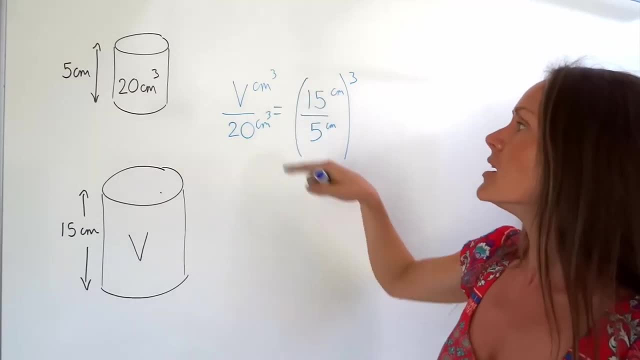 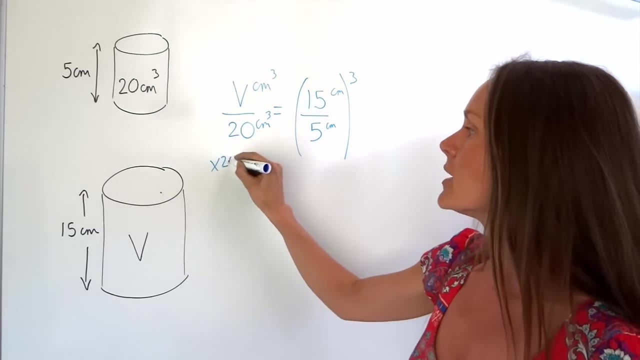 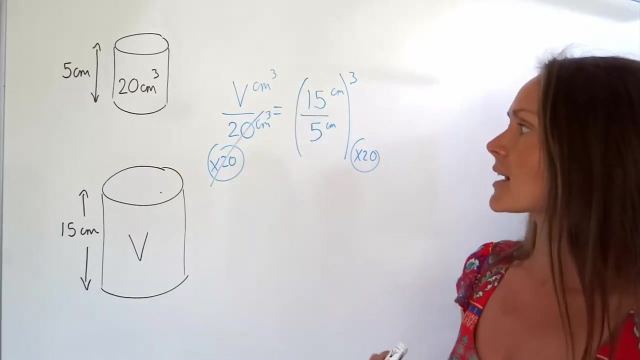 that it corresponds with our answer units over here. so the next step in solving this equation is to get rid of this divide by 20, and the opposite is to multiply and remember when you're solving you need to do exactly the same thing on both sides of the equations. so on the left hand side that cancels and 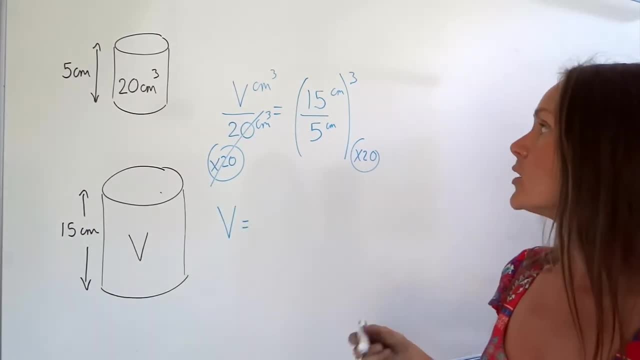 we're left with the volume V and on the right hand side we need to calculate. so you've got that fraction from earlier- 15 over 5- and we have to cube that one. remember to turn those centimeters into centimeters cubed- and then you will multiply that answer by 20, so you can just pop that in. 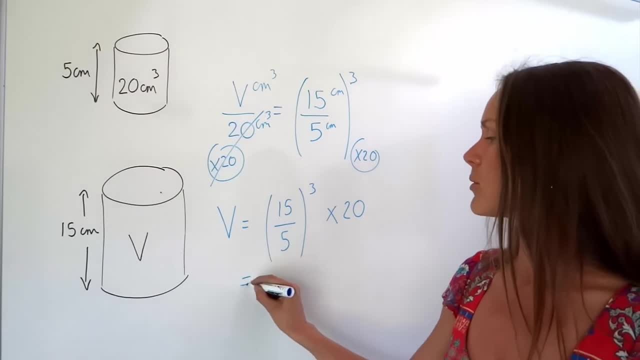 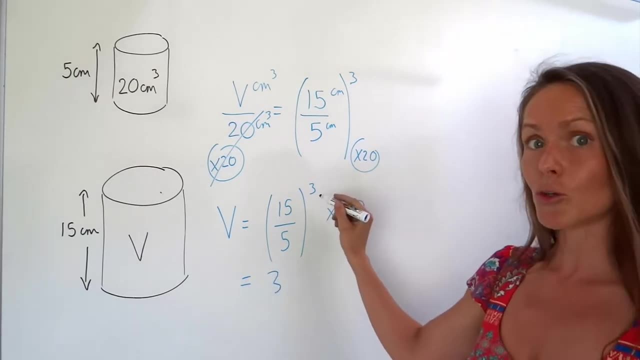 the calculator. I'm going to have a go at doing this in my head because I don't think it's too tricky one here. so I've got 15 divided by 5, which is 3. don't forget we've got to cube that number. and then I have to multiply by 20. 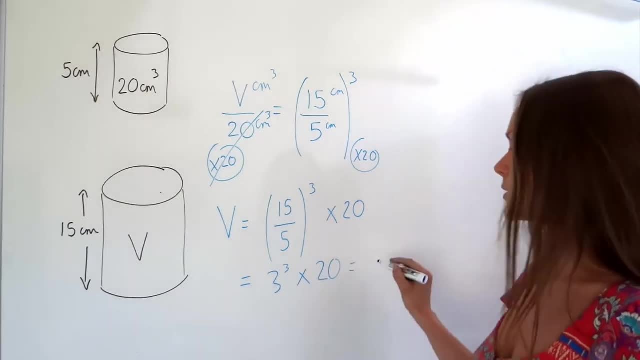 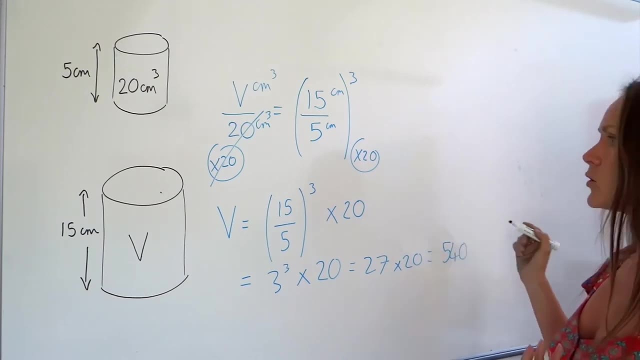 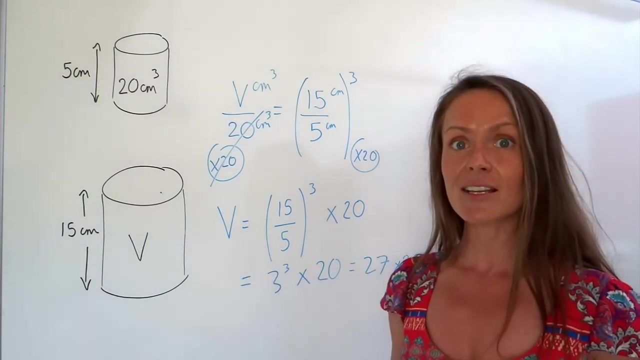 well, 3 cubed is 3 times 3 times 3, which is 27. then I need to multiply by 20, which gives me 540. not forgetting the units, it's centimeters cubed. so I've worked out the volume of the larger cylinder. okay, on to example number two. 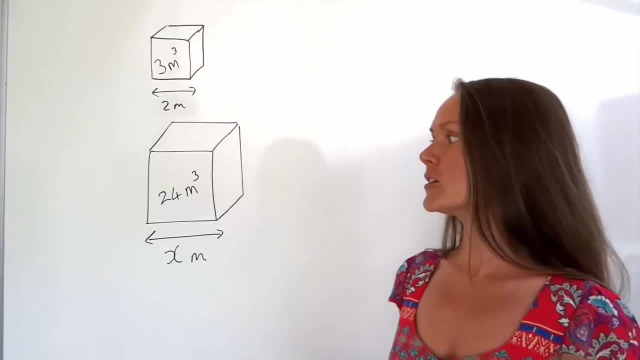 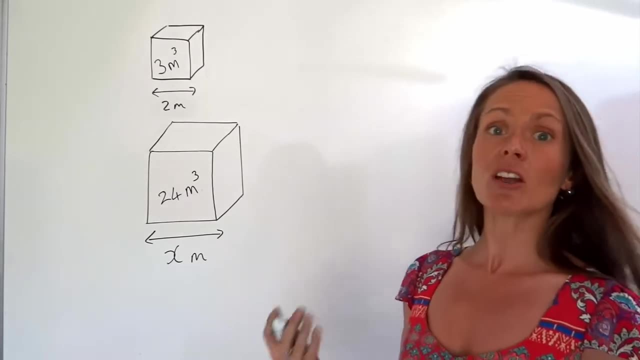 ok, so here's another volume question, except this time I know both the volumes, but I need to work out one of the lengths. this one here, X. so we're going to start exactly the same way and I'm going to write down unknown. so I'm going. 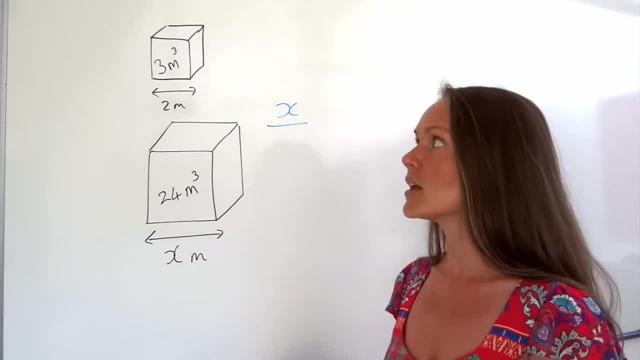 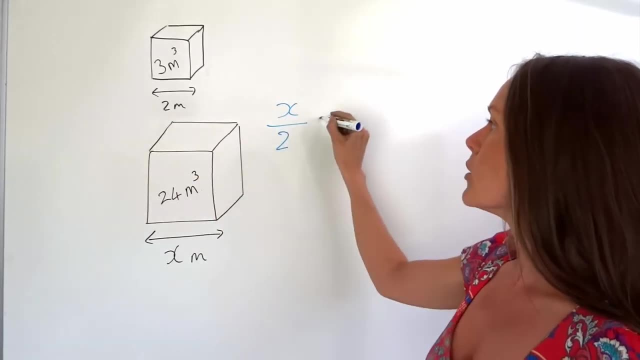 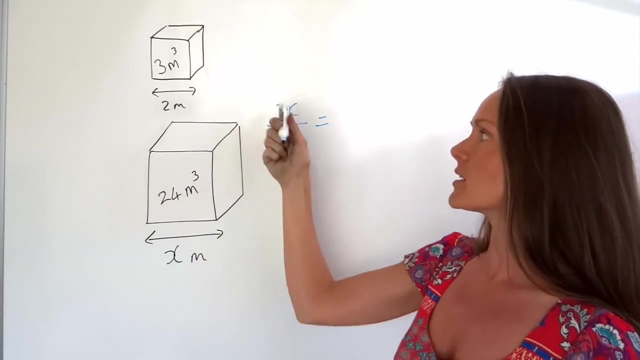 to write down X and I need to divide that by the length in the smaller cuboid. so I'm going to do the large length here divided by the small one, remember. you then need to divide the volume in the same way. so, remember, we've got the large cuboid as the numerator and the small one underneath. 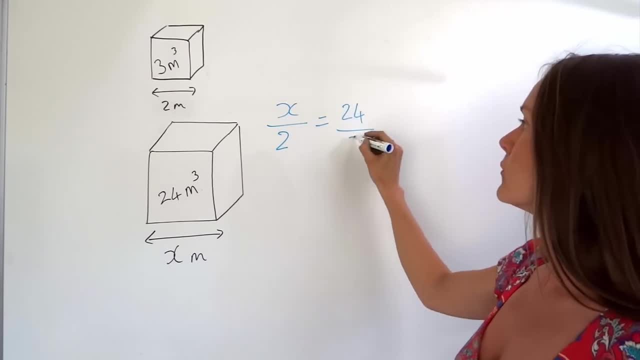 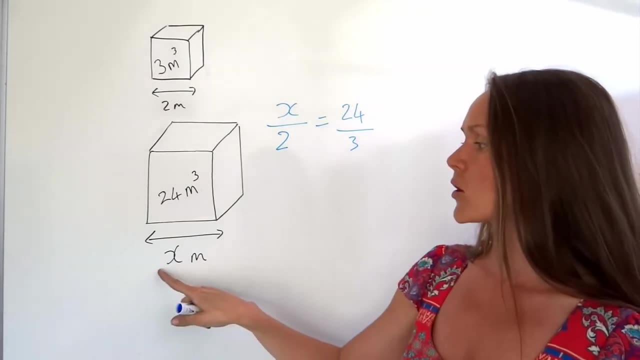 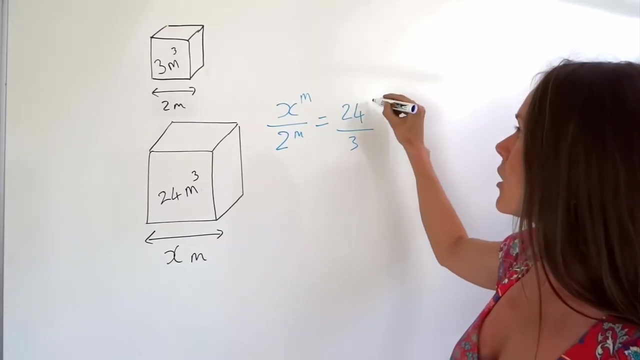 So I've got the large volume on top and the smaller volume underneath. So, just like before, we need to look at the units of our answer, And our answer is going to be in metres. Well, this length is already in metres, but these ones are volumes and they're in metres cubed. 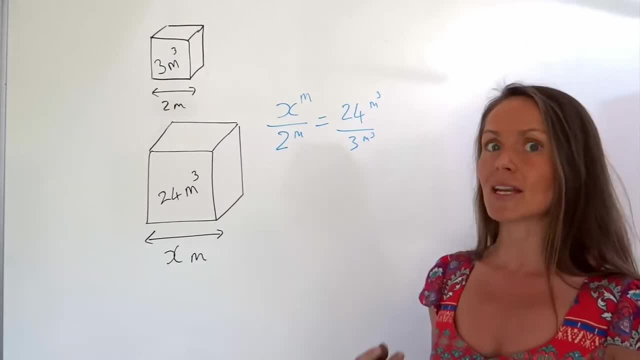 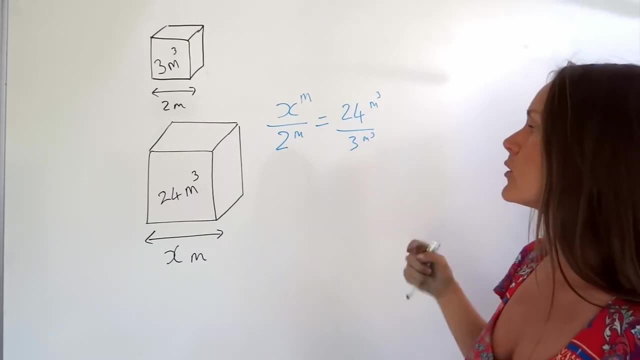 We need to make sure all the units are like the units in our answer, so in metres, before we can solve the equation. So we need to get rid of these cubes over here on the metres cubed. So the opposite of cubing is cube rooting. 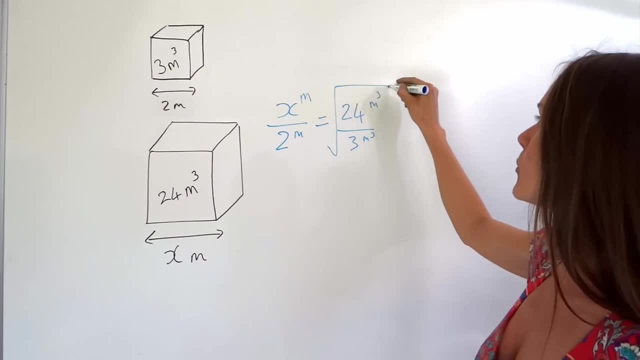 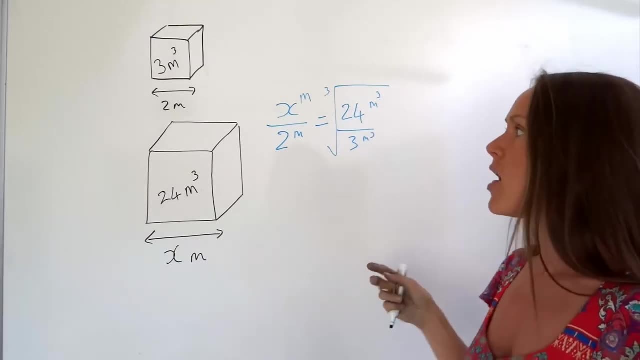 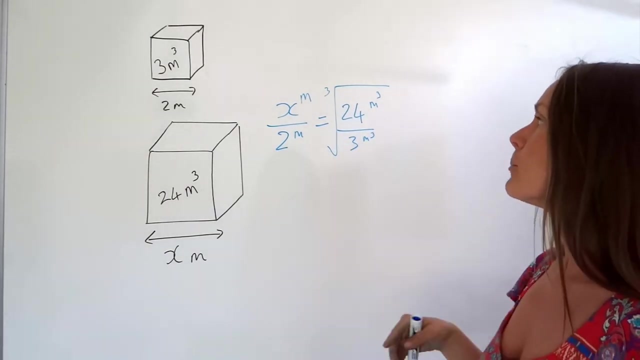 So to get rid of these cubes you need to cube root the right-hand side, Because there that will cancel the cubes and you'll be left with metres. Then everything will be in metres and you can solve the equation. So I could simplify here: 24 over 3, but I'm just going to leave it like this. 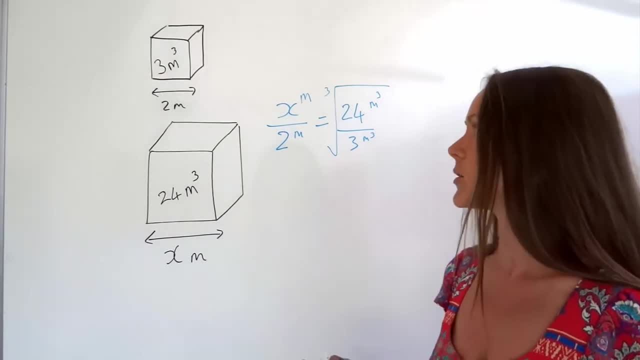 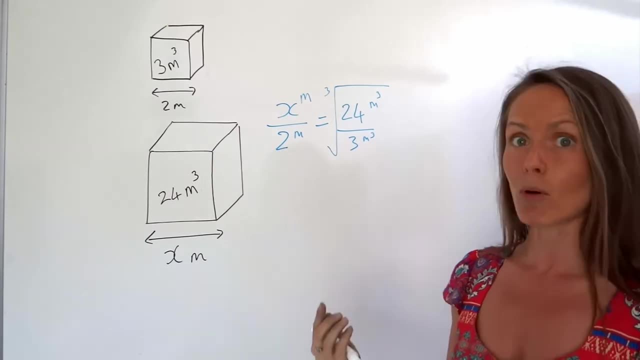 just so you know what to do when the questions get a bit harder. So what we need to do next is get rid of the denominator. So the opposite of dividing by 2 is to multiply by 2.. So I'm going to times by 2 on both sides of the equation. 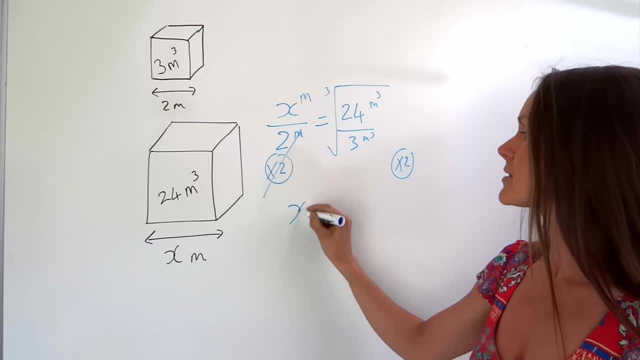 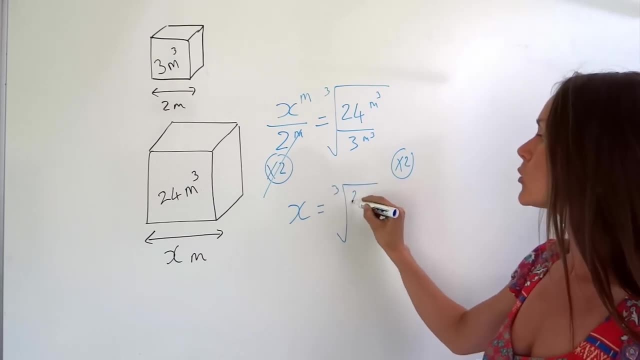 On the left-hand side that just cancels and I'm left with the length x And on the right-hand side I need to cube root this answer. remember So that big fraction. Make sure you cube root all of it and not just the numerator when you put it in. 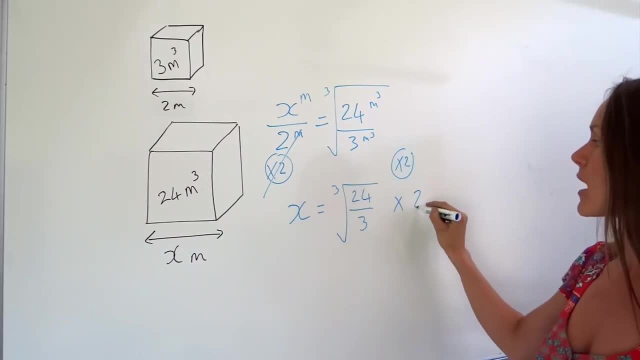 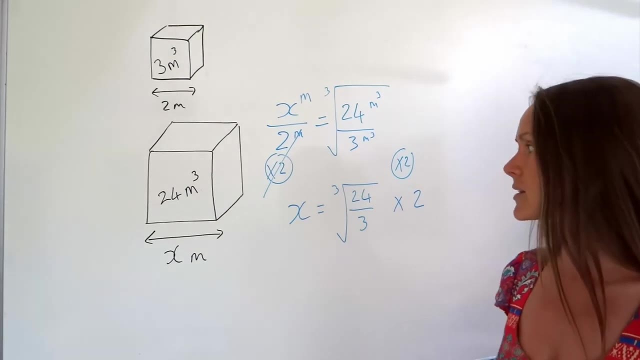 your calculator And then, not forgetting you- times all of that answer by 2.. So you could just put that all in the calculator and that will work out the value of x. I'm going to have a go at doing this in my head because I think it's quite an easy one. 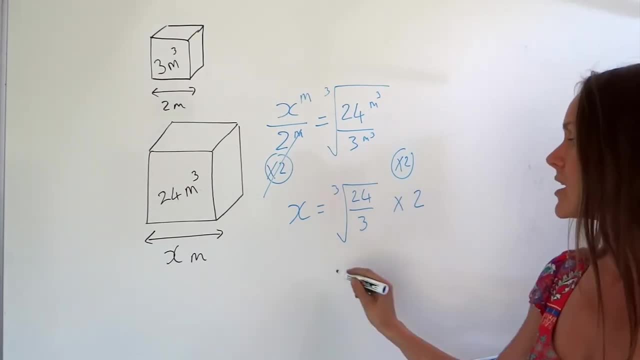 So 24 divided by 3 is actually 8.. So I'm going to change that fraction to the number 8 and I need to cube root that number before I times by 2.. The cube root of 8 is 2, because 2 cubed is 8.. 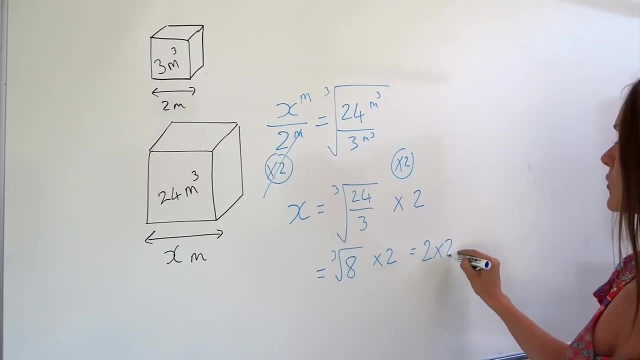 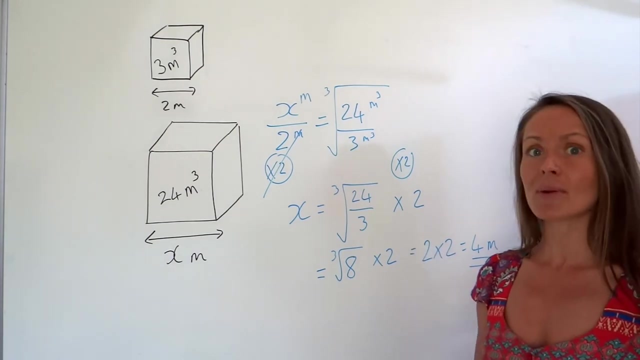 2 times 2 times 2 is 8.. So I've actually got 2 times 2, which is 4.. So the length of that larger cuboid here is 2 meters. Oh, 4 meters, sorry, Okay. so there are two examples on similarity and volume. 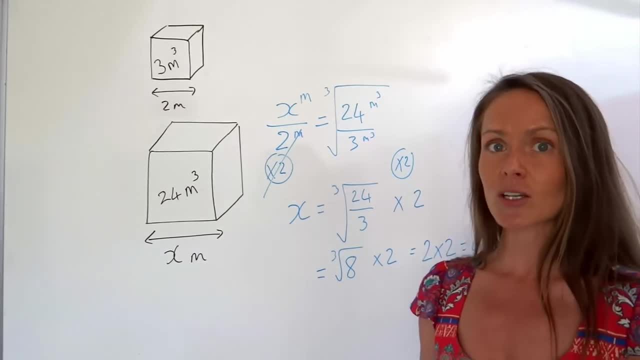 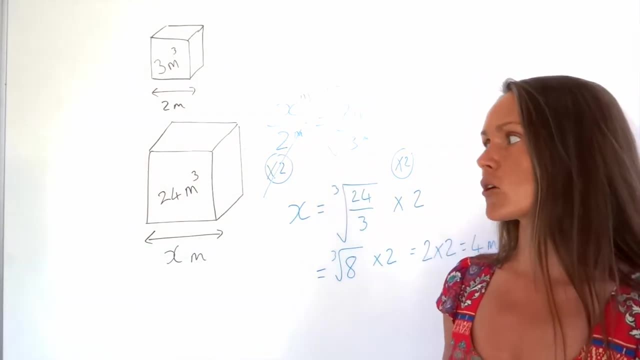 Soon I'll have some videos where I'll have a go at some exam questions with some challenging questions on similarity and it might be a combination of area and volume in the question You might need to cube, root, then square to make sure, just like in this example, that 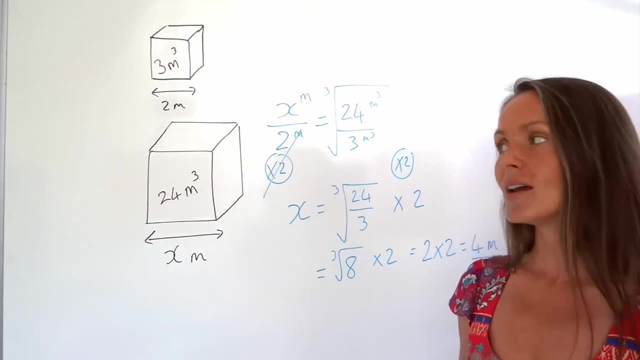 all the units are consistent before you calculate the unknown. So I hope you understood that video and that's bye-bye from me.